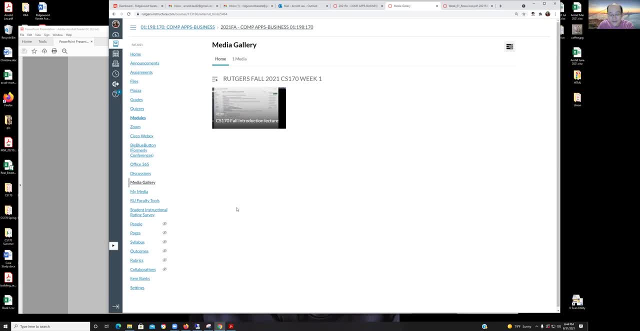 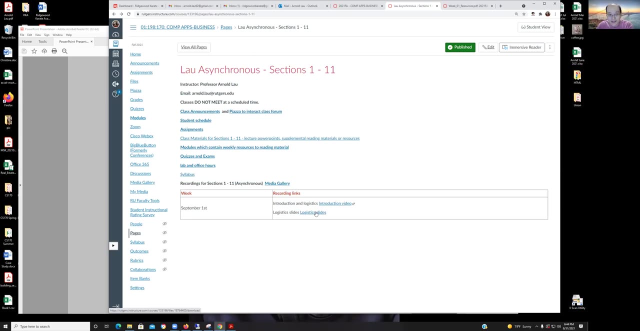 if you, if you see something that's interesting that you might find useful, Okay, so let's. let's go back to here. So the other thing I also put in here is the logistics slides, And this is kind of covering, like, all of the different sections for CS 170, not just mine, So pretty. 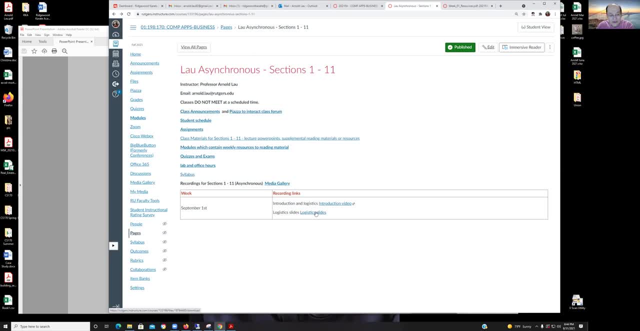 much covers what I covered. The only thing that I noticed that I missed in there, which I'll kind of mention here, is the idea of free lates. So free lates, you have one free late, And what that means is that you remember I was talking about when you submit your assignment late, that you're going to 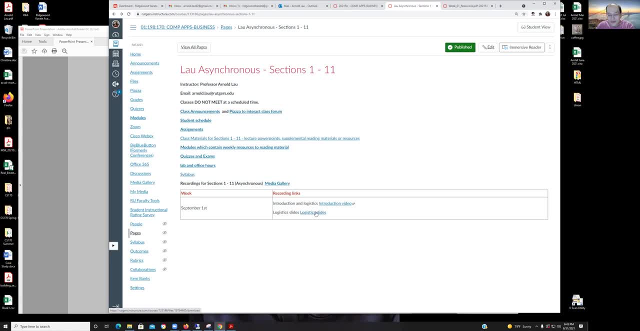 get 50% off your grade. So with the free late, as long as you tell myself and your TA ahead of the normal do day that you're going to exercise your free late, then you can submit it by the submitted date as of submit by date and then you won't lose 50% off. but you have to make sure you let 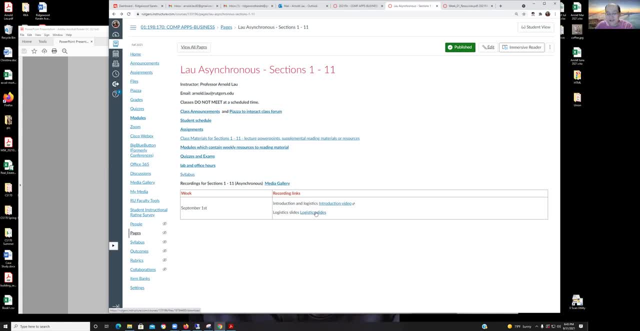 us know before the original due date for the assignment. Okay, so be mindful of that, And if you want to just refresh, go ahead and take it. these look logistics slides, But, like I said, I think I covered all of this material. 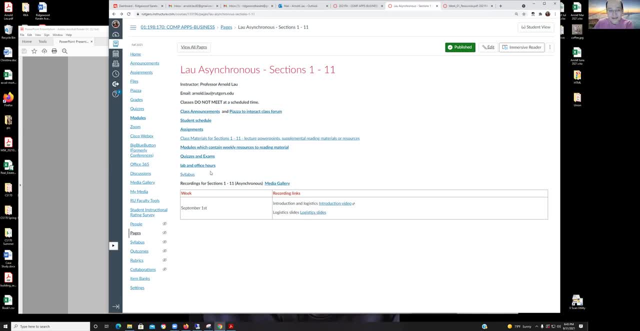 So, just as a reminder, in the article you can see it's the first video that I uploaded and I uploaded it And I'll just go ahead and take a second and refresh it and you can see it's actually the first one that I said I uploaded. So before you guys start going online to download it, you 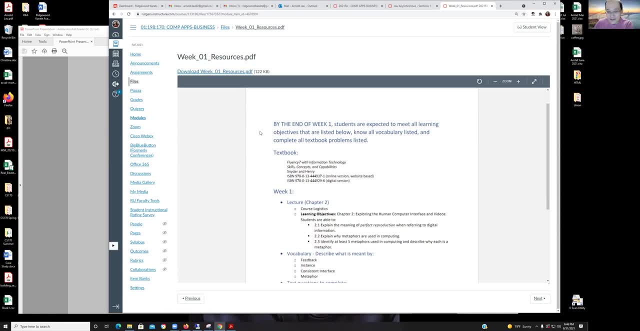 can click on the way. I've put it in the chat box And I'm using it right now. if you don't know this, you're using it. Okay, now let me go back to the slide deck. Where was I talking about? 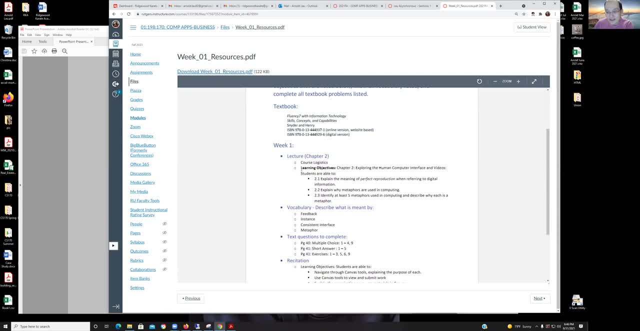 We're still here. Okay, here we go. Okay, learn what's our learning objectives. So you'll see, we have chapter two. What is all these different things here? And then what's going to happen in your recitation? So this is kind of like maybe. 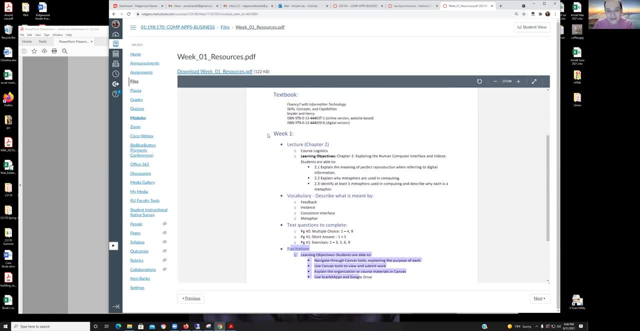 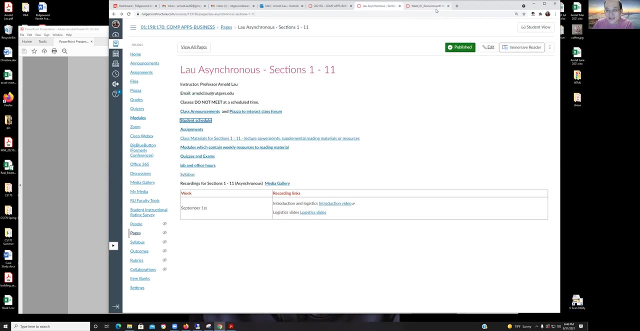 just giving more details to what you see on your student schedule, which is what I mentioned over here: the student schedule. Oops, that was a syllabus. Let me get out of here. Where's the student schedule at? No, let me go back to here. I must have put the wrong thing in there, So 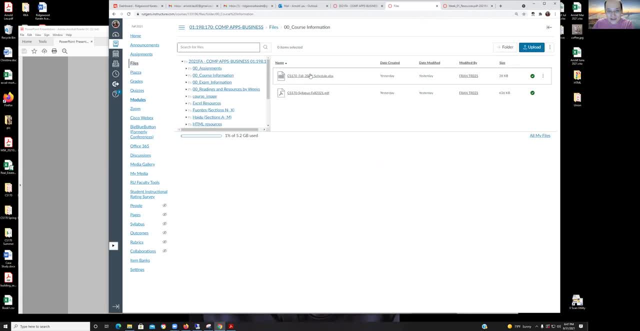 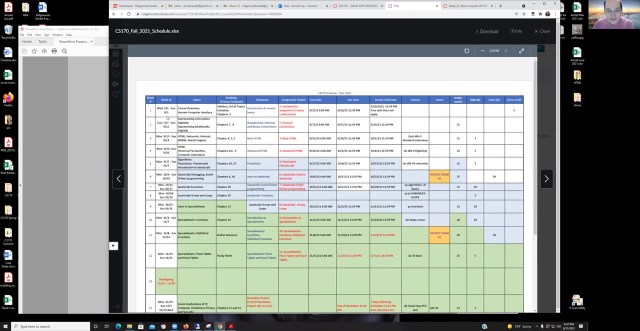 course information and student schedule. So I linked the syllabus in there aside, But anyway, you can see it's laid out. Like I said during the last lecture, it's laid out every single week what we're supposed to be covering, what the readings are. 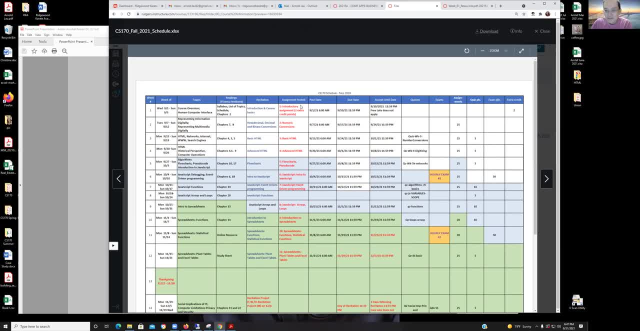 the recitation, the assignments- that's going to get posted. you know the due dates, you know the posted date, that's. you know the scoring. So you know. you pretty much have a very clear view of what we're going to be doing on any given week. Okay, whether it's looking at this, 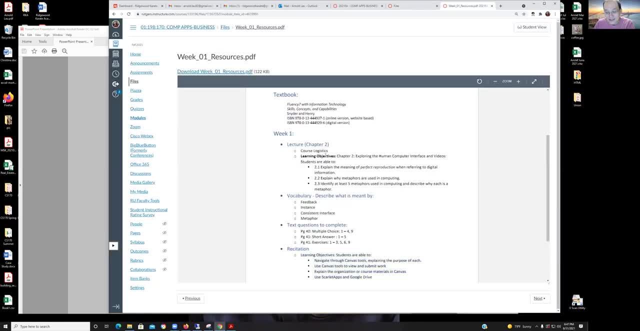 looking at the module, looking at the course, looking at the course, looking at the course, looking at the modules, like I said here, right, so kind of just gives you more detail than what the spreadsheet gave you. Okay, so it's something for you to pay attention to. Okay, So I can even see. 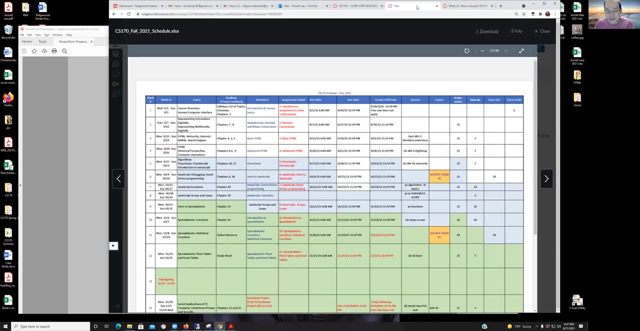 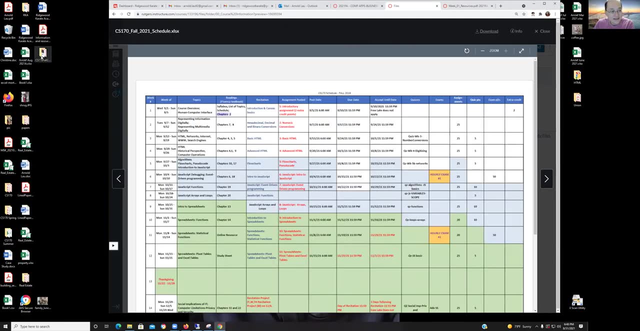 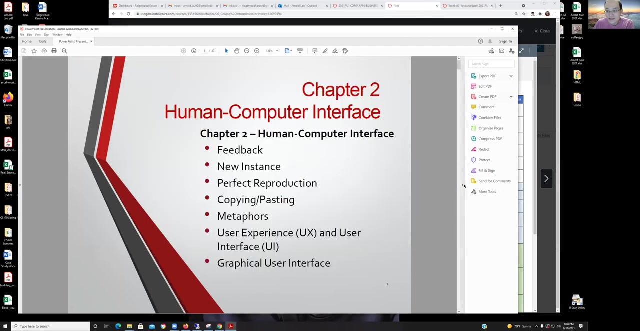 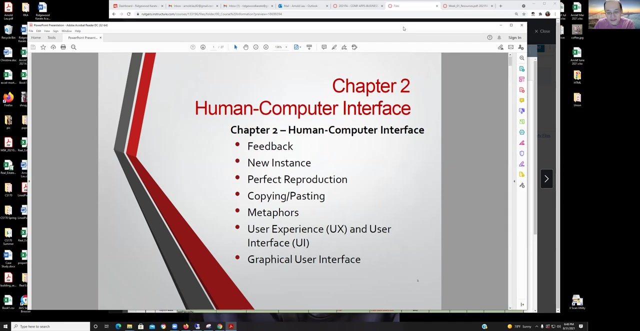 here you can see the lecture is talking about chapter two here, which lines up to here. chapter two, Okay, So see, here I'm gonna close this and let me get over to here And chapter two. Close this up here, Okay, And you know. so this first lecture is, or first week, it's basically a. 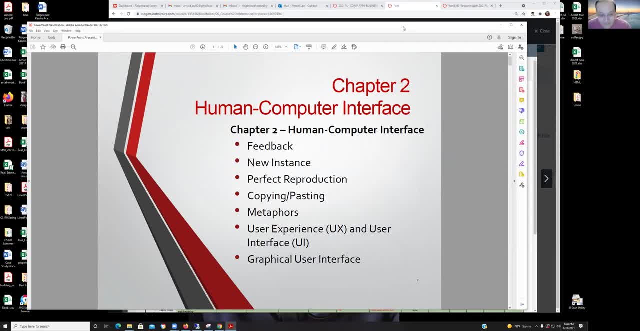 lot of students are going to be doing add drops, So not going to really do anything very, very heavier, complex this week, Because there will be students that may not show up until for class, until next week. Okay, And that's why your assignment this week is only an extra credit thing, So it's. 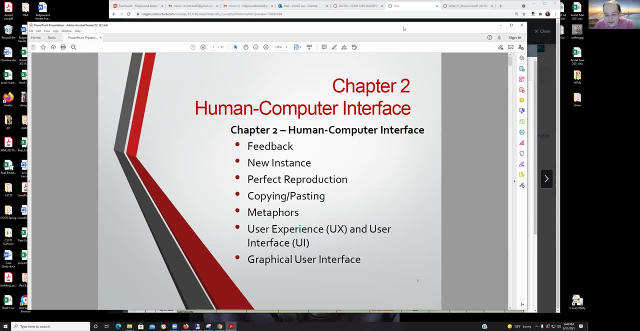 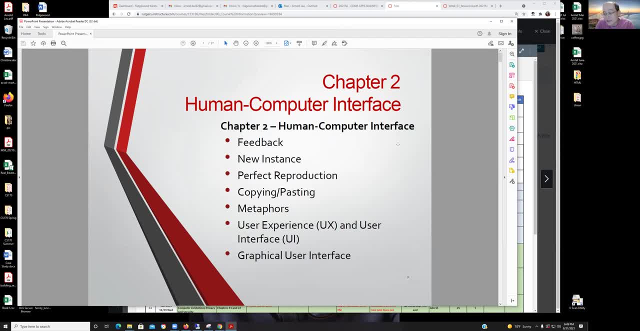 know the, you know the questions that we need to address. So a clear, real clear picture is kind of all of the hard focus that we're we basically clear to, to give a包括 a, not just a final pitch. So if we, if the broadest of our questions, are gonna do theneck option This, la do an. 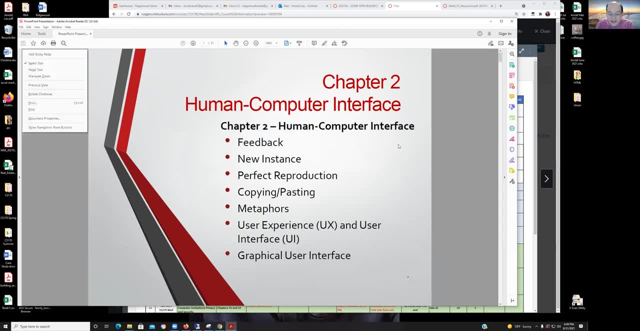 toolkit, So I think, in a landscape study, maybe you you could just tell me: uh, what do you think of this project? Well, yeah, so, so this background application will actually be internal classes. andrée begrudgenerateigen Ma monitoring data. right, So no, not easily. So light pencil, So not. 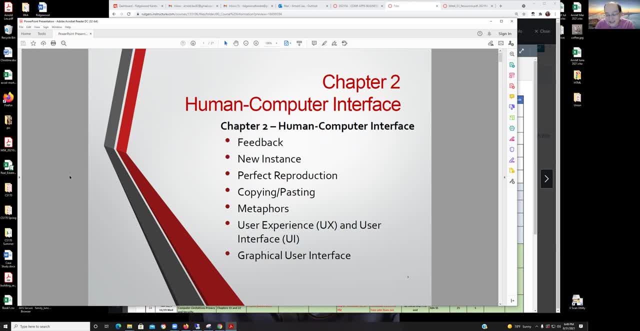 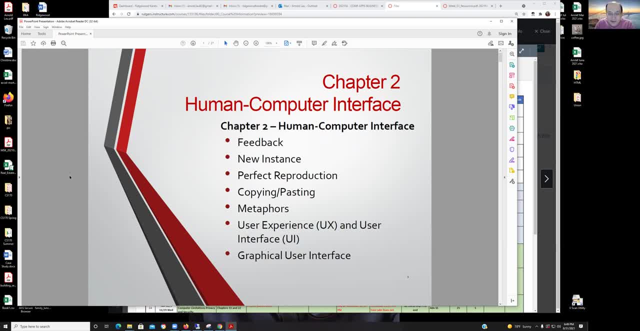 for the exam. okay, um, so you can take it for what it's worth, right? so what i'm gonna go through? i'm gonna probably read through this, um, but, like i said, you're probably best served to make sure you just read the textbook on this, take some notes on this stuff and use that as part of your. 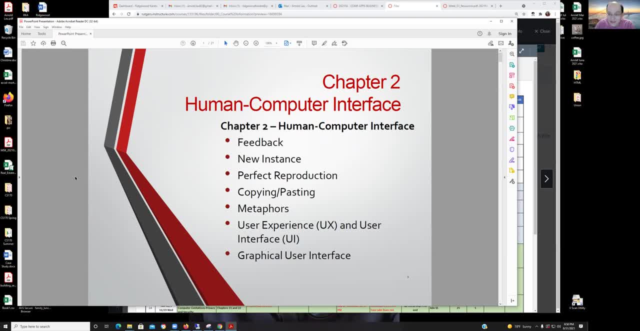 your notes that you'll use for your exam. that comes up, okay, and we'll probably ask you some questions sort of like: yeah, you know what do we mean by feedback, what's some examples of that and stuff like that? so it's kind of that type of knowledge for this chapter too. all right, so i 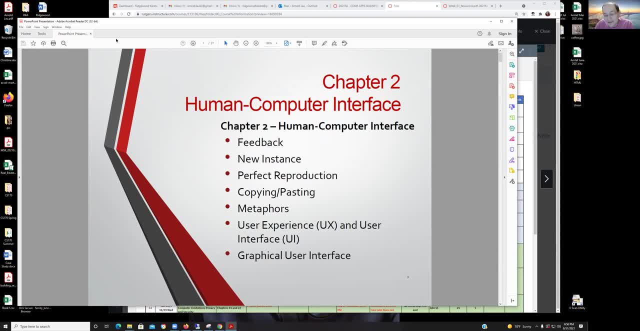 won't spend too much more time on it. but, like i said for this aspect of the um course, it's one of those things that read the book. it's one of those things where we can kind of brainstorm and and book and make sure you understand that the points being made in a book and just take some notes and 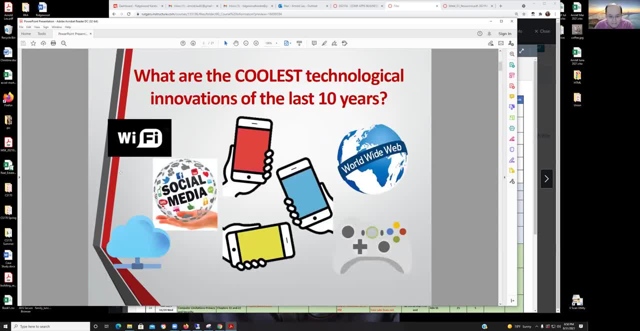 refer to it for your exam. Okay, You know. so this is basically just talking about all the things that you probably have in your daily lives, right, You know? whether it's like your mobile phones, you know, accessing Wi Fi, doing stuff on the internet, social media. 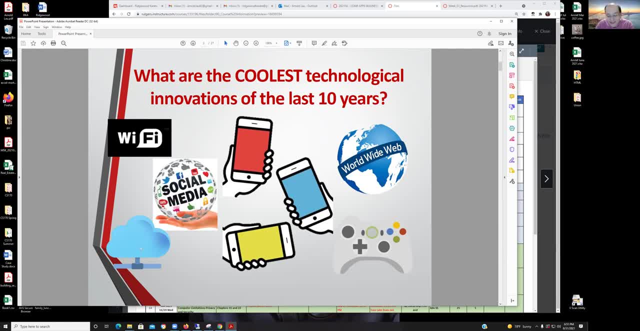 doing games- I guess this is supposed to be like a cloud, So doing stuff on the cloud. you know all the pictures that you take, you know upload to the cloud and whatever right. So that's kind of like the different things that you know. it's probably commonplace for most of you. 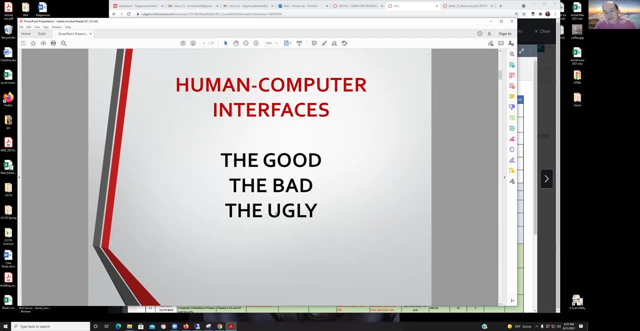 Okay, So human computer interface is really just talking about how do you interact with your, with your computer, right? I mean, there's many different ones, You know. if you look at, you know probably the most common ones right now. probably most people are accessing. 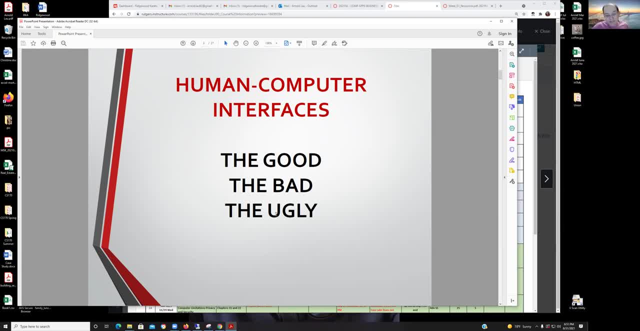 their technology via their phone. Okay, Who knows what it may be in the future. Maybe it's more and more on the voice side of things, Maybe it's virtual reality, Who knows? But as of right now it's kind of very. everything in terms of interface is very driven off of, like the mobile. 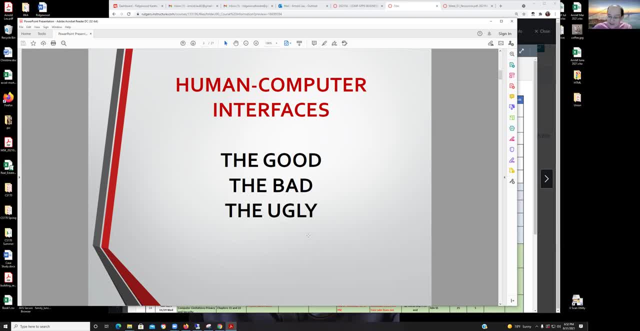 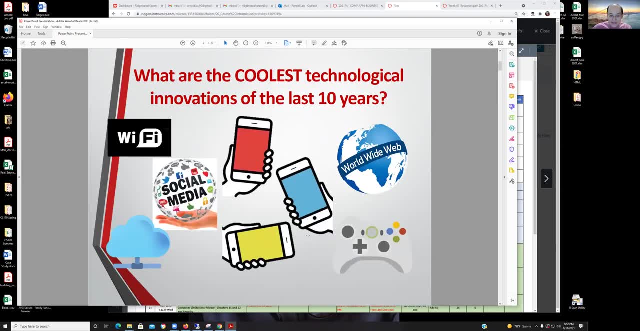 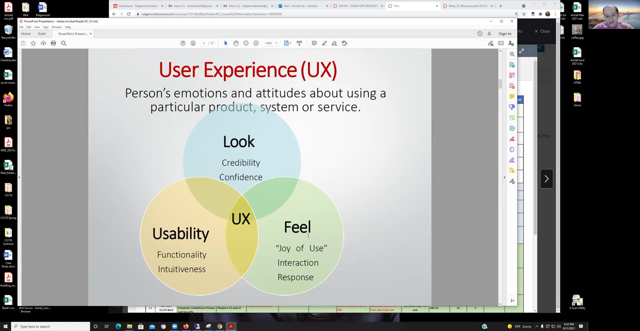 platform. Okay, But you know it is almost going to be like a history thing, right. We'll kind of go back into the past history of computers, how they developed, And you know we'll see how we got to where we are now. Okay, So one important concept here is the idea of user. 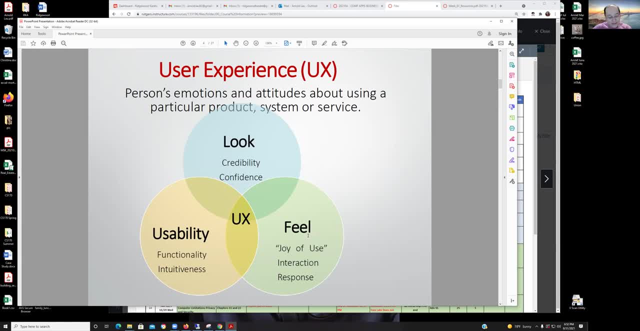 experience right, And you, you all know this right. You know the people that are very successful with this from a commercial standpoint would be, you know, people like Amazon, but there's others too- And it's the overall user experience And that's the, that's the, that's the. 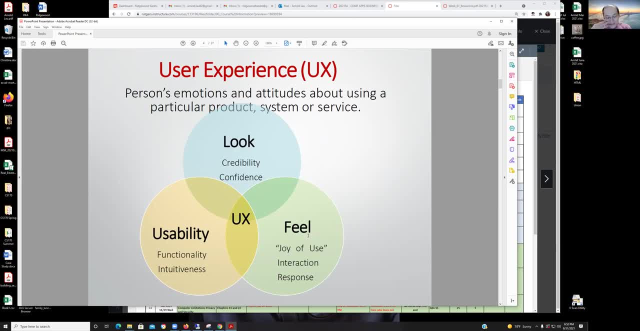 kind of actually even drifted into like the, the bricks and mortars world too, right. So taking you know someone or your customer, let's say, and how do they engage with you as someone who's offering a service or selling a product, And how do you feel when you come out, the other end of 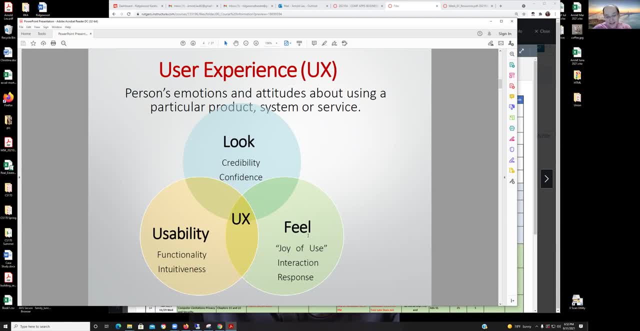 this process. Do you feel good? Do you feel brand loyalty, You know? are you feeling happy to spend more money on your product? Are you feeling like you're going to be able to make more money on your product? Are you feeling like you're going to be able to make more money on your product? Are 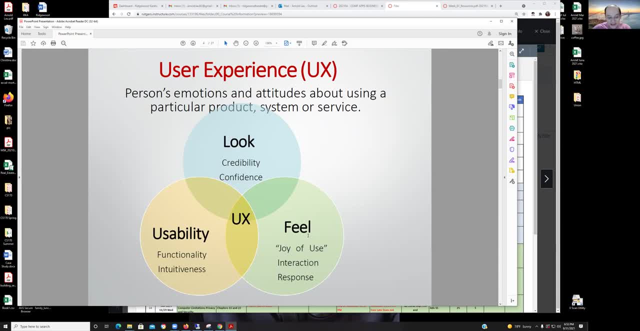 you feeling like you're going to be able to make more money on this product or continue to support this company, whatever, right? So it's a very big thing with user experience, right? And if you look at history, you know the user experience has come a long way. It was very clunky at the beginning. 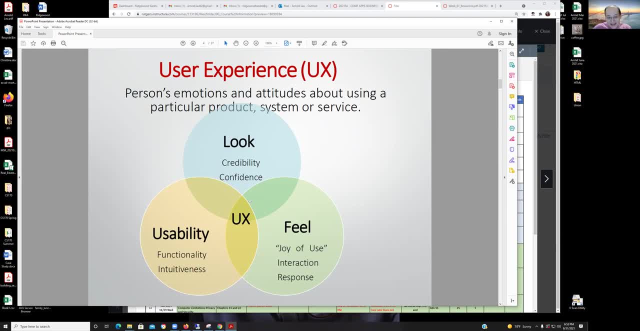 and a lot of people were just feeling their way around And now not to say we've reached perfection or anything like that. but you know it is a lot smoother, right, You know the idea of like in Amazon, the idea of one click- right, You know it's a lot smoother, right, You know. 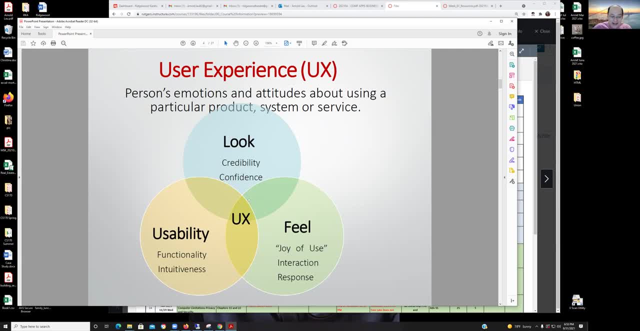 if you make it hard for someone to buy your product, even if you have a great product, you may not get as many customers as you would like. right? People have a very short attention span, especially these days, So you know they don't really have that much patience for a clunky. 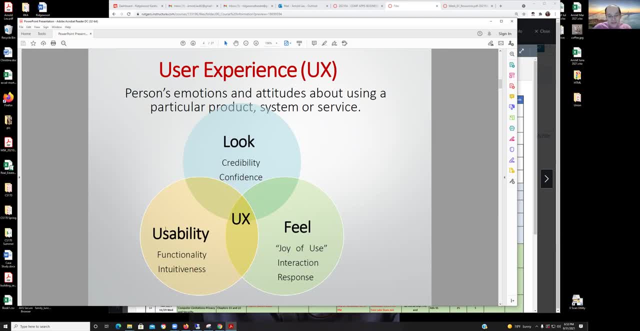 user experience, right. So this is Venn diagram and this is kind of sort of something that you're going to see in the future. So you know, if you make it hard for someone to buy your product, actually when we go into like searching for different things on the internet, and I'll get. 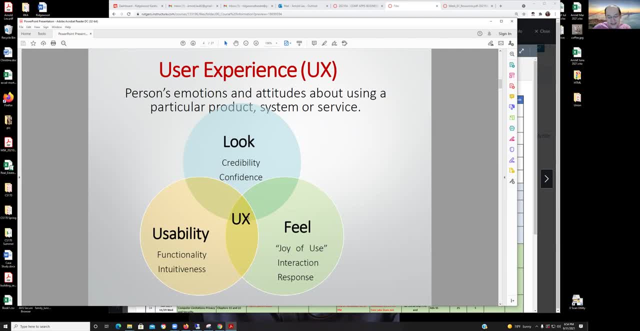 to that later. okay, So you can see, UX is sort of like the intersection of all these different concepts here. okay, You know, if you see something just like when you do writing right, If you see something with all kinds of different weird fonts or spelling mistakes, 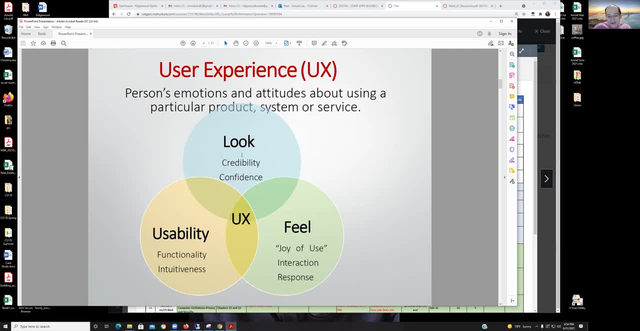 or laid out hard to read. stuff like that you don't really think that's really professional, right? You know, back in the days before you had like all these you know products to make your stuff look slick, you know people would do it by hand, or 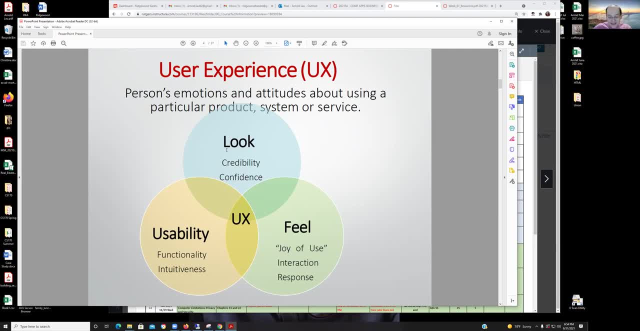 you know, come up with their own formats for things. It was very easy for things to just not look professional. It looks kind of amateurish, right. But these days there's a lot of tools that basically package things up and you just have to put in some content. 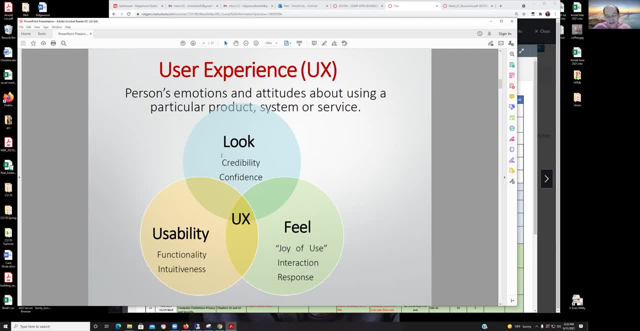 and then it just makes it look very slick and professional, right. So you know that type of thing: if it's not looking that level of slick and professional, it just makes you look like you're, you know, amateur, basically right. So that part is. 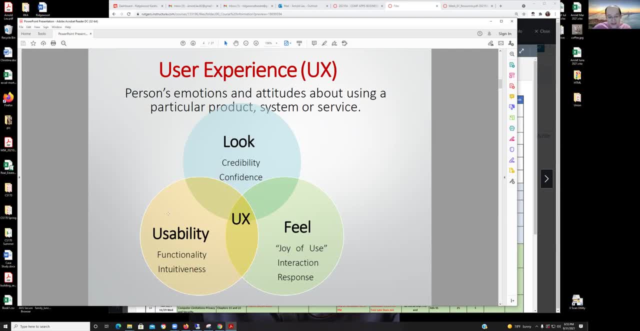 you know, kind of self-explanatory right, Usability right. I kind of think of it in terms like what are the capabilities, What can it do? And intuitiveness right. So you know I can tell you personally if I go to you know I can tell you personally if I go to you know. 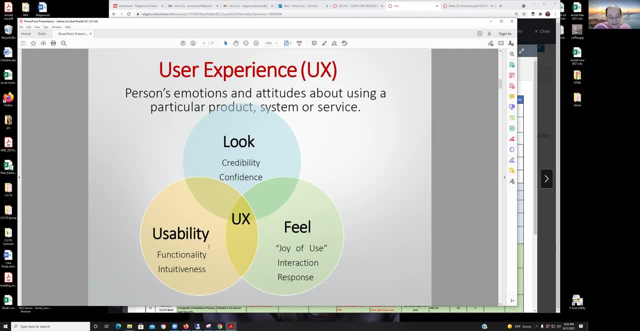 like deal with, uh, you know, paying my bills on on like the electric company, or, um, you know going to like the township website to pay my property taxes, or this or that water bill or whatever. most of those interfaces are horrible, right. the usability is absolutely atrocious, right? uh, they obviously. 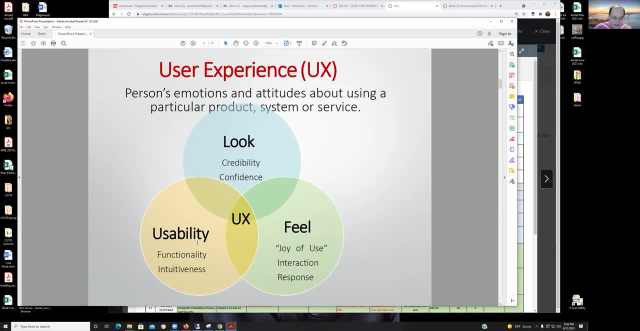 don't have much experience from the likes of, like, uh, what you're used to, let's say, on amazon, where you can look at your past history of purchases, um, and it's very intuitive. you don't need, like you know, any training. you don't need, like any, like user manual to figure out how to use it. 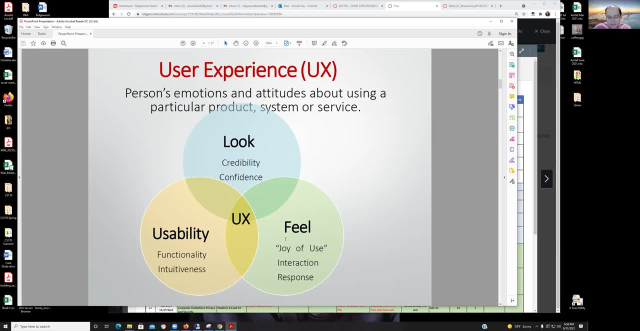 all that type of thing. so usability is there and just the overall feel right, you know, is it like, you know, you click on something, you don't have any feedback, you don't have any understanding, like are they doing anything? you know, did your transaction go through? uh, those type of things? okay, um, you know, and i'm sure if 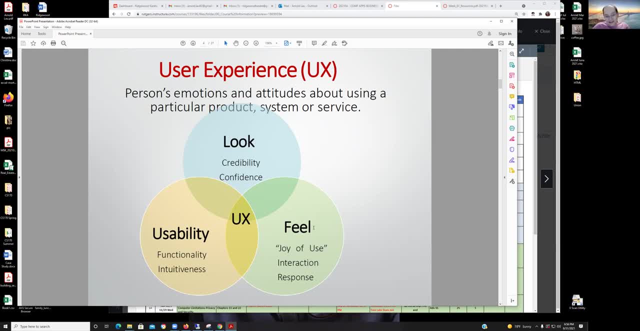 you think about it, you'll you'll kind of have a good feel, based on, probably most likely, your e-commerce interactions, on what is a good user experience. right most places now, if you don't have a good user experience, you're probably not going to be successful as an e-commerce. 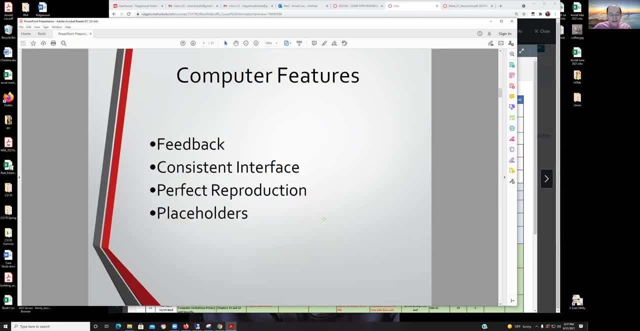 setup. okay, uh, so part of what feeds into that? well, feedback, right. so if i click on something, and let's say it takes a long time to process, right, and i just click on it and you don't see anything. you don't know whether the computer is doing something, you don't know whether there 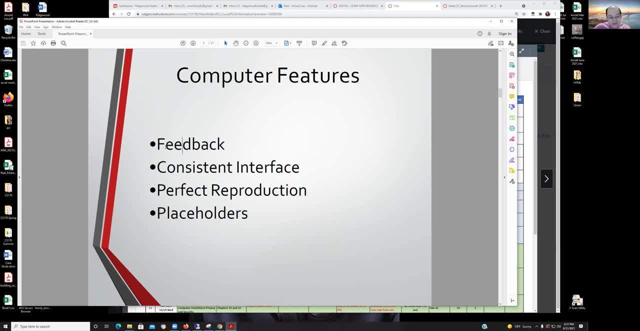 was an error. uh, you don't know when it's going to get done. nothing, right? i don't think anyone likes that. right, you're probably sitting there, you probably end up clicking it multiple times or whatever, right? um, you know, just like when you go into elevator lobby, right, you know people hit. 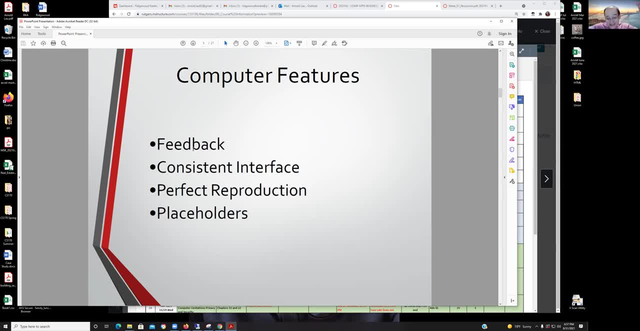 the elevator button. they like to see like the elevator bank, they like to see the elevator with the number coming down. they, they all, say oh yeah, the elevator is going to be here soon. um and uh, you know, knowing when it's going to come doesn't make coming. it make it come any faster. 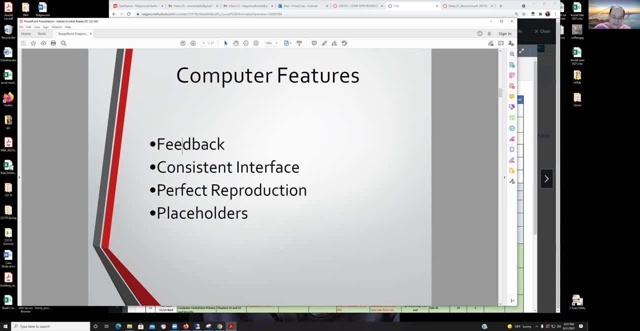 uh, but having that feedback mechanism, uh, sort of like you know, addressing that feedback mechanism is really important, right? so if you look at, you know, on a computer typically if something's going to take a long time, maybe you'll see like a progress bar that kind of shows how far along you are on downloading something, maybe. um, whatever it is right, maybe even. 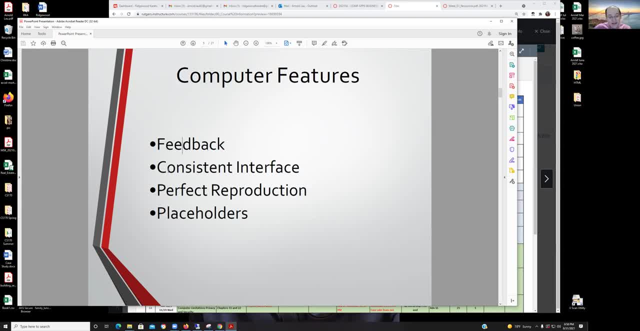 how far you are in a movie or something, right? um so, consistent interface: right. if i learn how to use one part of, let's say, microsoft office, um, hopefully, because there's a consistent interface, i can use the other products of microsoft office fairly easily and i just use microsoft office because you know it's one of those pop. 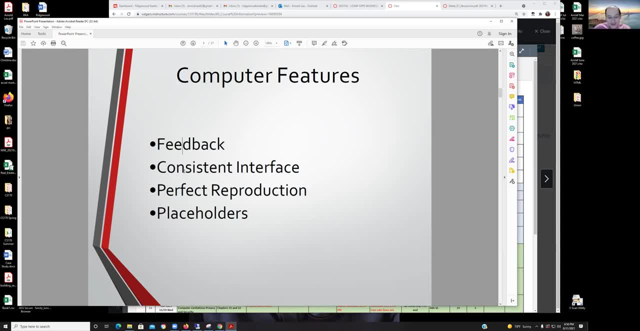 common things that a lot of people use. especially, we have a free license for it here at rutgers. so consistent interface. uh, perfect reproduction, you know, being digital. there's this idea of like: um, you're able to, and it's digital means zeros and ones. right, you can perfectly replace that. 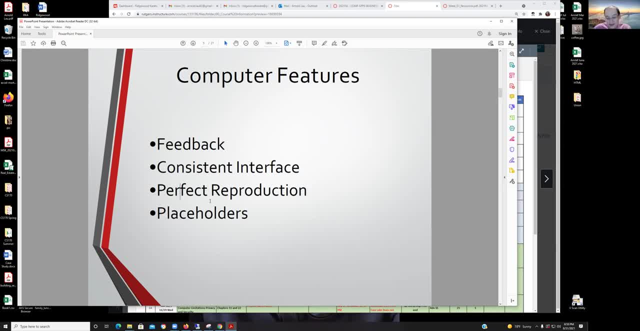 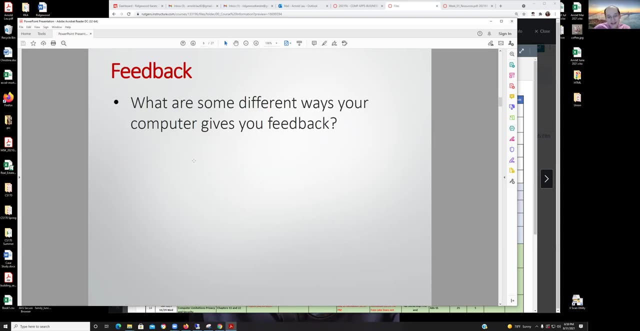 reproduce that right. that's pretty easy, as opposed to analog, which, you know, over time, the copy uh will eventually degrade, okay uh, and placeholders, okay uh. so we'll come back to these, uh, hold on in a second right. um. so, like i was just talking about what are some of the different ways. 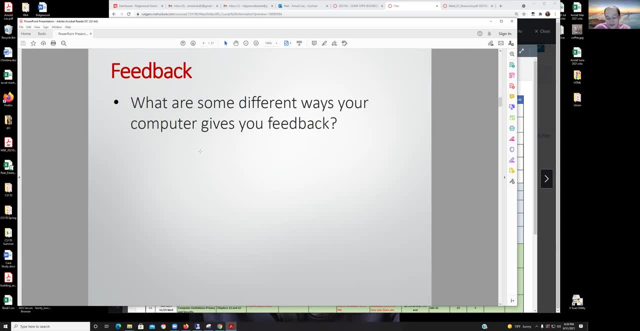 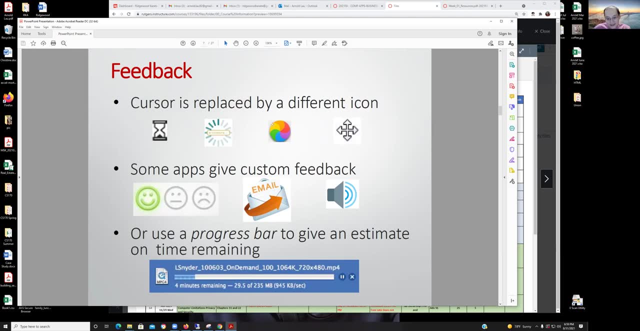 that your computer gives you feedback, right? i mentioned it before the progress bar, right, so you can see that here. hourglass, you got processing, you got this little spinning uh kaleidoscope thingy. um, you know you have this directional thing going on here. um, you know you have these different things here. 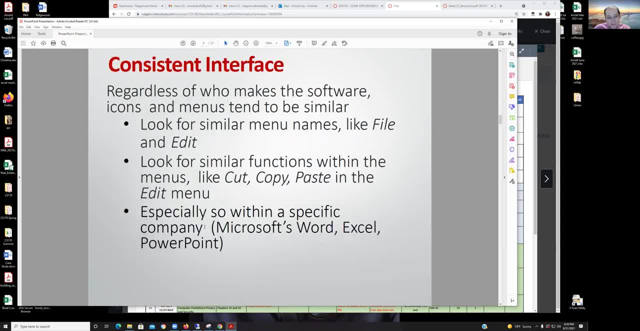 like i mentioned before your progress bar. okay, consistent interface, right? so, like i was mentioning for, like microsoft office, you'll see things like file and edit. uh, you have similar types of things, right? um, and you could trust in different things like, uh, it's available in different ways, uh. 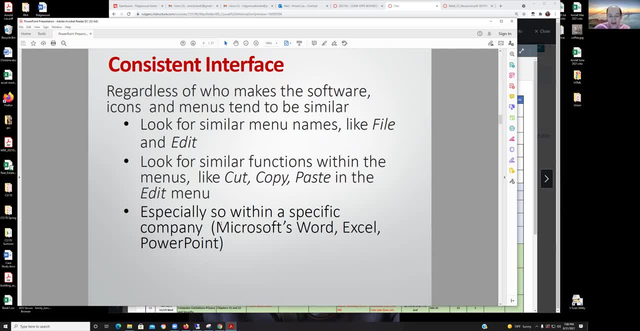 screen reader and things like that, uh, but you don't have to get really into the different things. it's also similar to something that you can like paste on different things, right, um, and you know, like i alluded to microsoft office, uh, which includes word excel, powerpoint, among other. 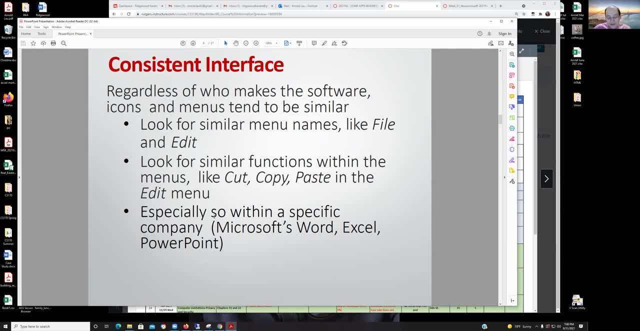 things. um so consistent interface. it helps in terms of training, right. you don't have to like learn something totally different for something that's not even necessary. it's not, uh, you know, let's say, Word versus like Excel. right, You're saving a file to the file system. 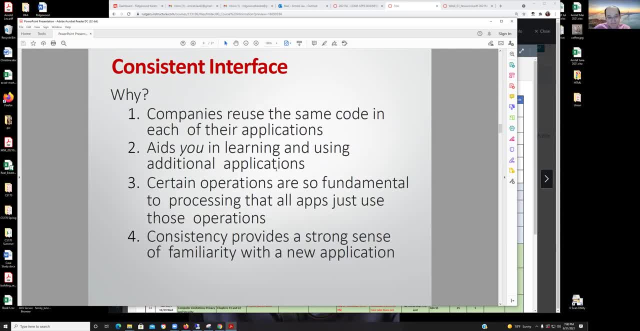 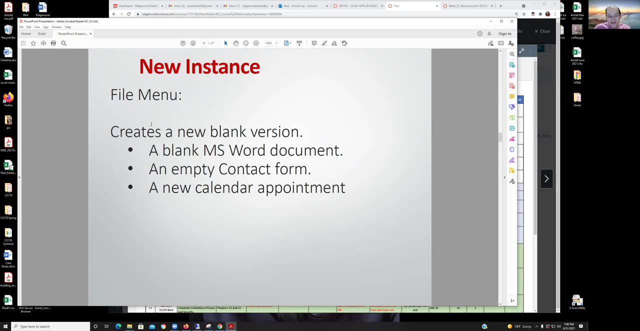 do it the same way and do it consistently, right. And so, like I just mentioned, there's sort of different reasons why you would have a consistent interface. okay, You know a new instance, right? This would be like basically creates like a. 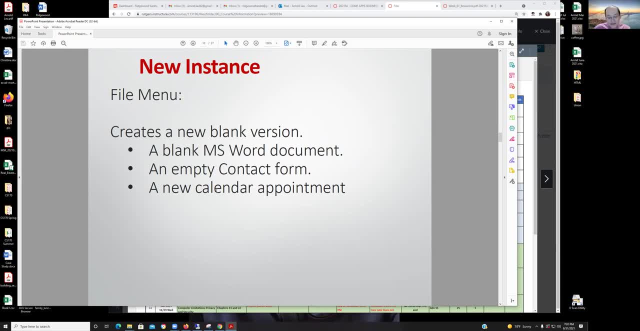 let's say, a new Word document, right, A new contact form, new calendar appointment, right- And just creates a blank version of it. okay, But again, this is part of a consistent interface, right? This is just a behavior that happens across all of these apps. 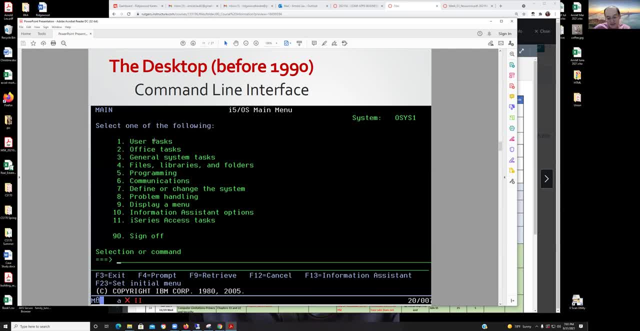 All right, this is just an example of really a mainframe interface. You know, I doubt many of you have seen it, unless you work at some of these, like retail, these old retail chains or whatever, like PC Richards or something like that. 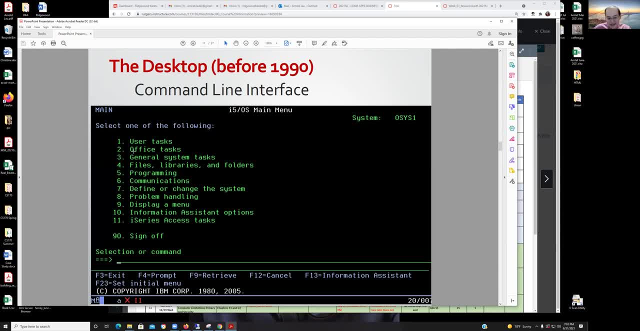 They still have their systems on the mainframe. So you'll see screens like this, right, So it's really text-based. So you're typing stuff here, you hit like a number and that's your menu option, right? So you like, you hit that number. 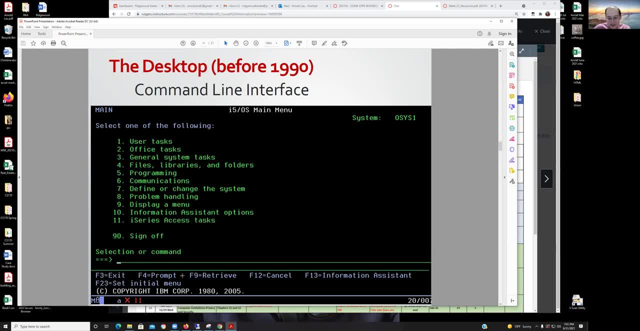 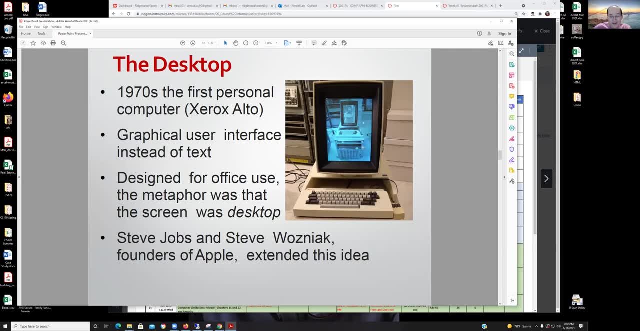 or you hit this F keys right At the top of your keyboard And then you step into, like you know, essentially from a personal computing standpoint, the idea of, like a graphical user interface or GUI. okay, Now, this is an important point here. 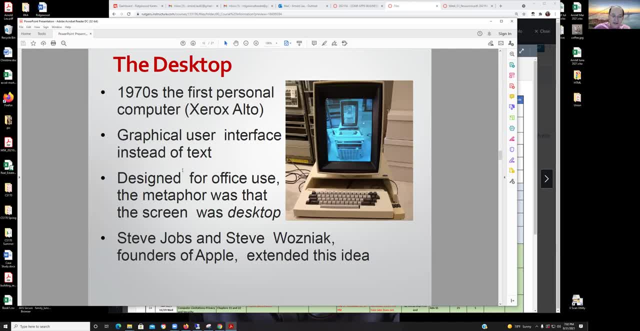 So pay attention. here There's the idea of who came up with this. who came up with this and who actually commercialized it, who bought it out? And then there's the idea of who came up with this. So the idea of who came up with this. 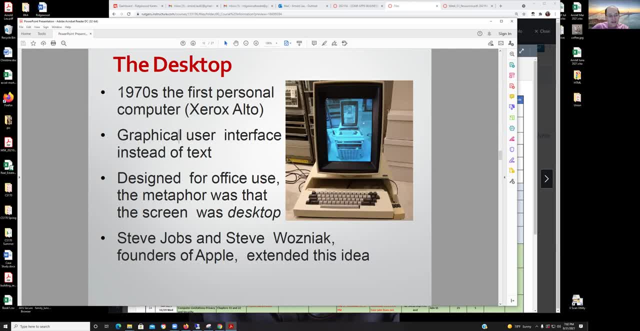 and who actually commercialized it, who actually bought it out, who actually made it out to market. It's two different things, right? And this team? this seems to trip up a lot of people, right? So Xerox is the first right. 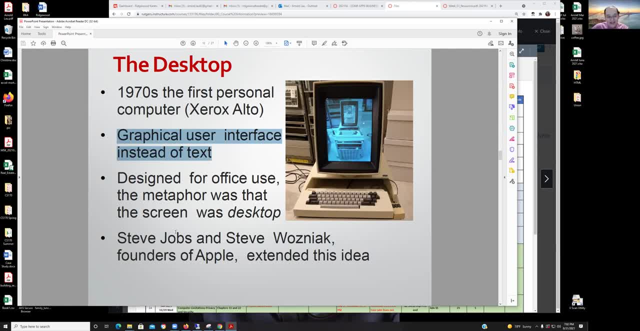 So they came up with it. So you can say they invented it right, But they didn't bring that out to the market, meaning like, oh, this is what Xerox invented, right. So that's why typically a lot of people think of Apple. 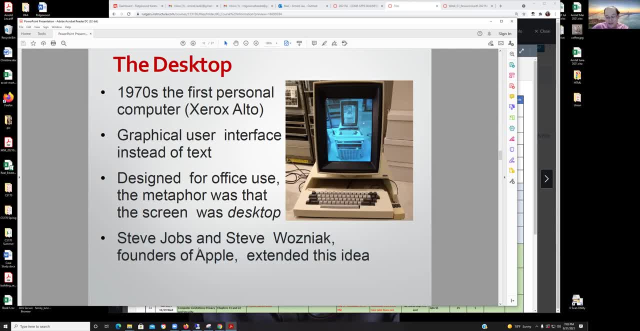 as the GUI and really you can say they pretty much commercialized the idea, but they actually didn't invent it right. So that's an important distinction And I highlight that because almost every semester I've taught this class that seems to mess people up right. 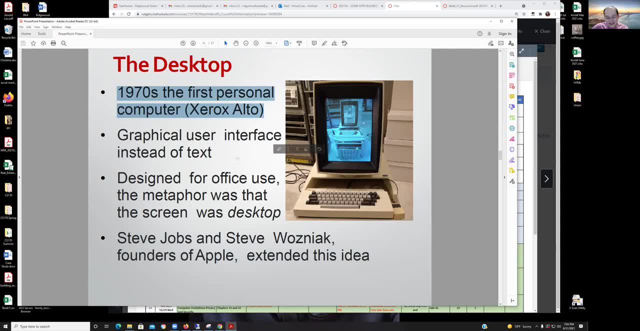 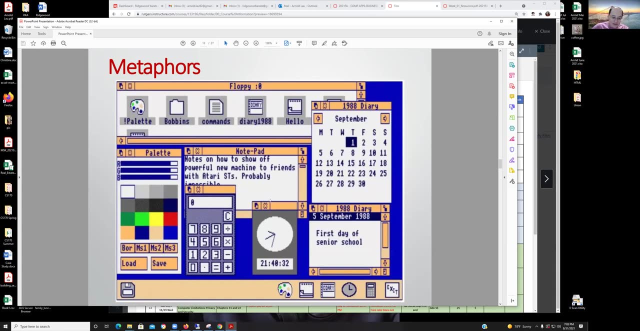 So pay attention, the difference between inventing it and commercializing it, okay, Or bringing it out to the personal computer market, okay. So metaphors- So in this case they're basically in this initial GUI- is the idea of you know. 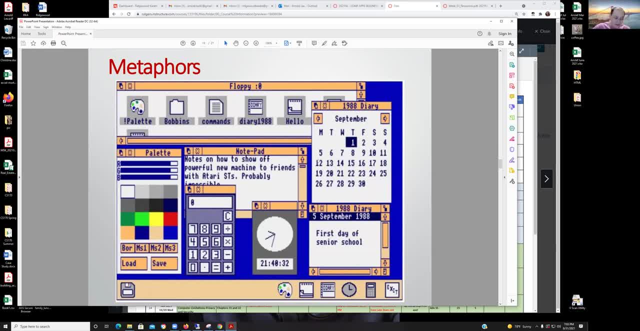 you're doing stuff on your desktop, right? So if you in the old days you were thinking about: okay, here's my desk, I would have a calculator on it, I have a calendar on it, I have a notepad, whatnot? 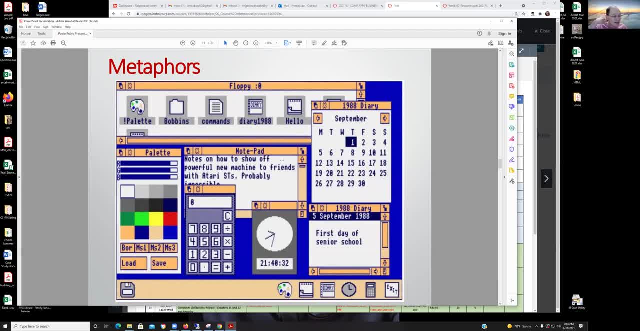 And so they basically created the idea of this desktop. on your computer, You would view it as a desktop, right? So that's what they mean by a metaphor, right? So the way you might open a file the way you might like, put stuff in the trash or whatever. 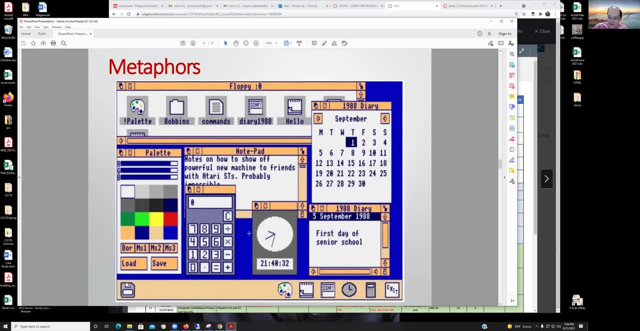 everything was kind of tying it back to what people understood in the real world, And it makes it easier for them to interact with the computer, right? So instead of looking at a computer and just typing everything by the command line and say, oh, open this file or find this file or whatever, 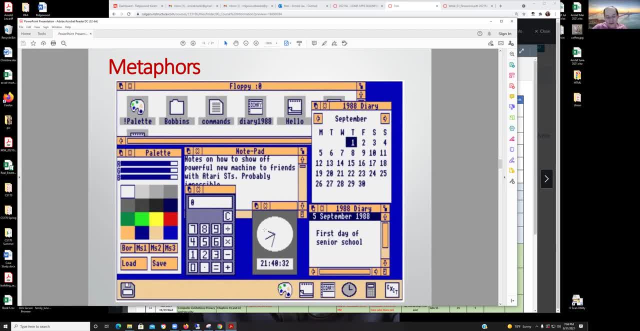 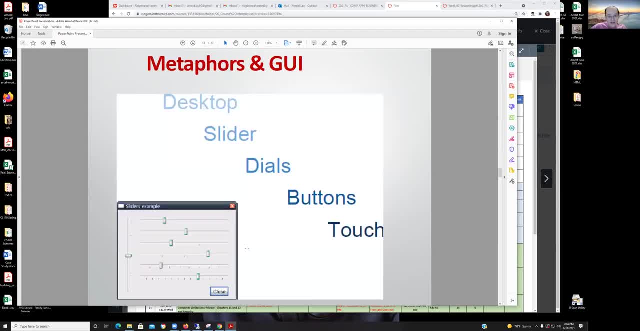 if I translate that and present it to you in a desktop form. that's a lot easier for the typical normal people to grasp onto. okay, And so you have these sliders and you have these buttons. you know it tries to draw analogies to like you know. 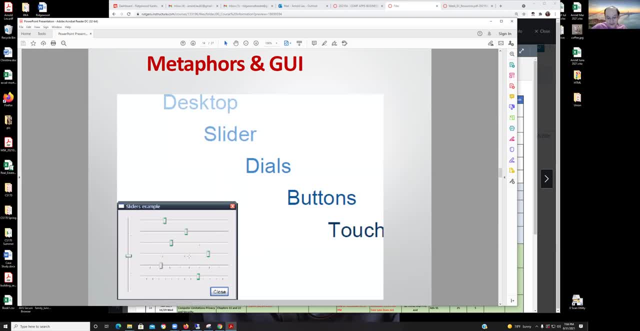 it tries to draw analogies to, like you know. it tries to draw analogies to, like you know, what you might've experienced in the real world. right, You know those sliders, I guess these days are probably not that common. 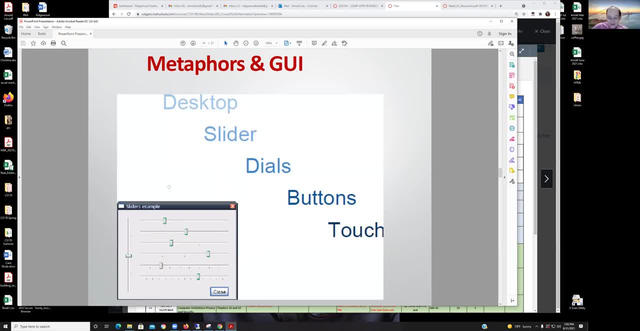 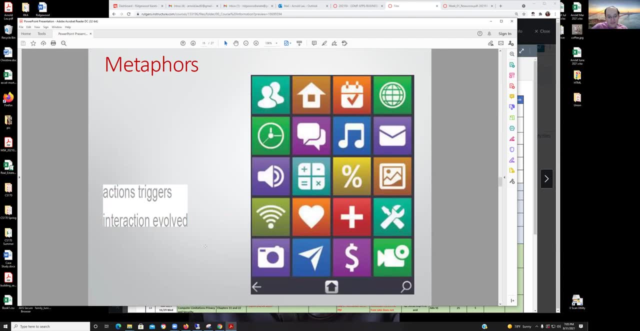 Back in the early days, sliders were very common on things like stereos and stuff like that. And so, looking at this, you know again, you're trying to look at things and see if it makes intuitive sense to you, right? You see a lot of things, ideally for things. 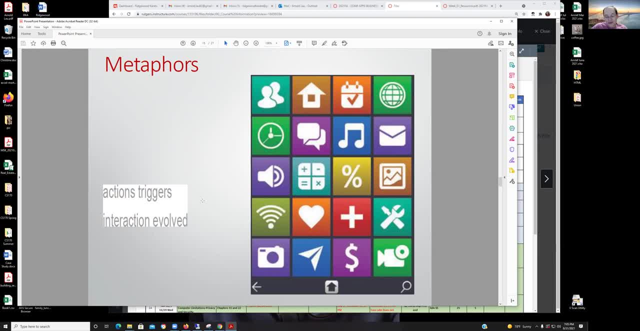 to work at the consumer level. you don't have to look for instructions, right. When you get your mobile phone you download an app. hopefully you don't have to look for instruction manual, right? hopefully it's very intuitive when, whatever app you download and you can work on it right. 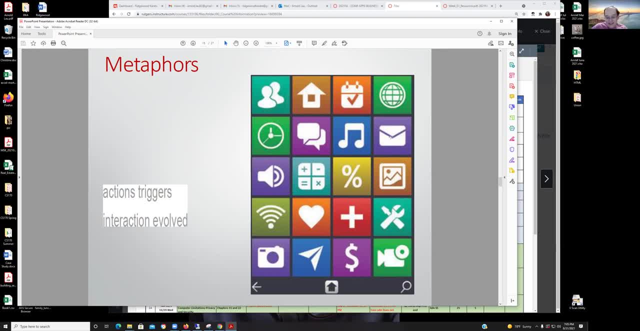 So if you see something that looks like an envelope, probably most people think of that as email, right? You look at this looks like some sort of internet connectivity. You look at this. this looks like a camera. right, This looks like maybe toolkit setup type of thing, right? 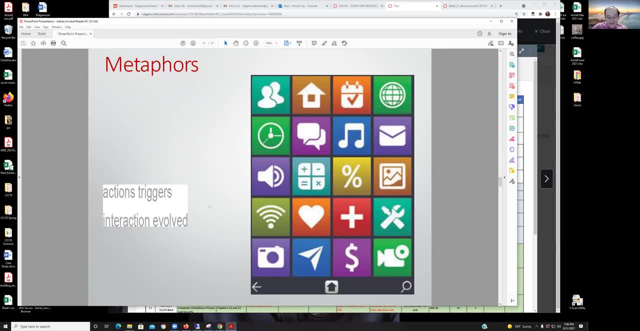 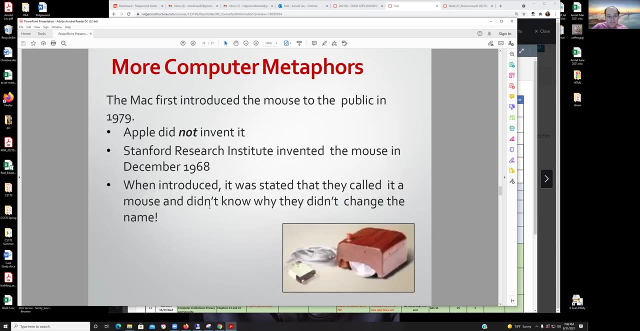 So, you know, that's kind of the idea with metaphors, okay, Trying to draw it to like a, you know, like something that the typical person can understand and interact with the computer in an intuitive fashion. okay, All right, so this is just talking about. 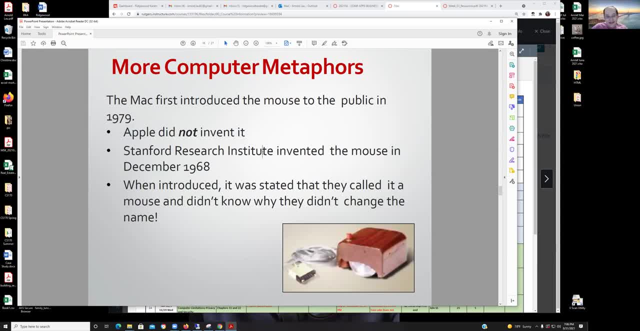 what I mentioned before, the mouse. Apple did not invent it, okay, All right, Yeah, so it's just like a little bit of a history trivia type of thing, right? Like I said, the only thing you wanna make sure you don't get tripped up on is thinking. 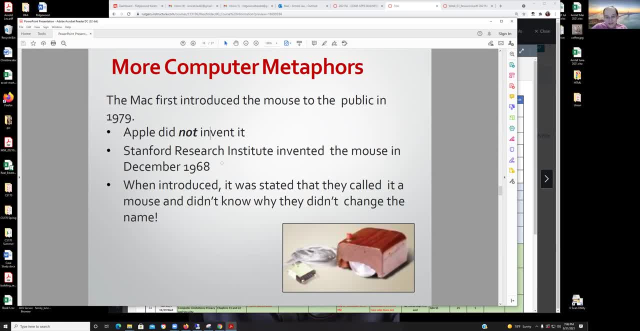 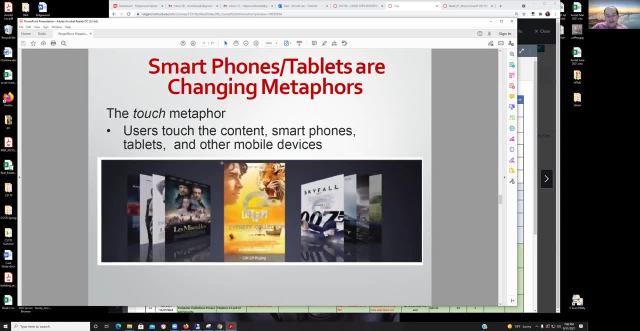 that Apple invented the mouse. okay, So just be careful with that when, inevitably, you're gonna be asked about that during the exam. right, So now you go into the touch metaphor. right, So now you go into the touch metaphor, right. 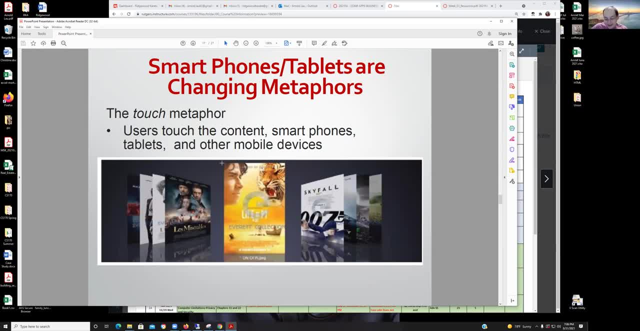 So now technology has progressed, You get all kinds of stuff. now that's gonna be on the mobile platform, And if you don't make your website or whatever you're doing on the mobile platform, you're gonna lose out on a lot of customers, right? 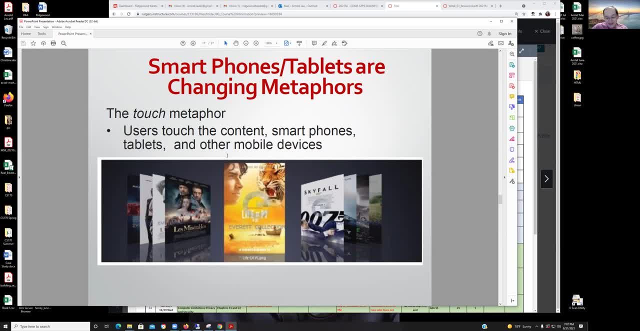 You know, I don't know what the percentage is, but at least 80% of people are interacting now through their mobile phones, right, So you really can't survive If you're just doing stuff off of like a website that's designed for the desktop and not mobile friendly. 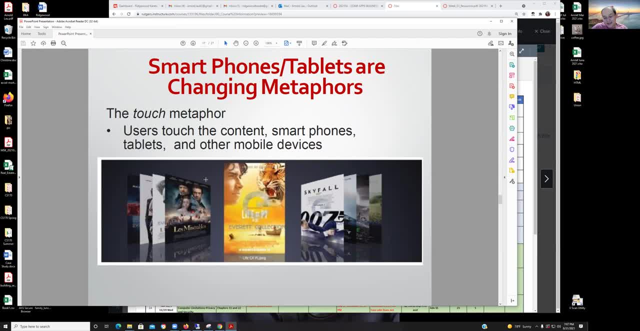 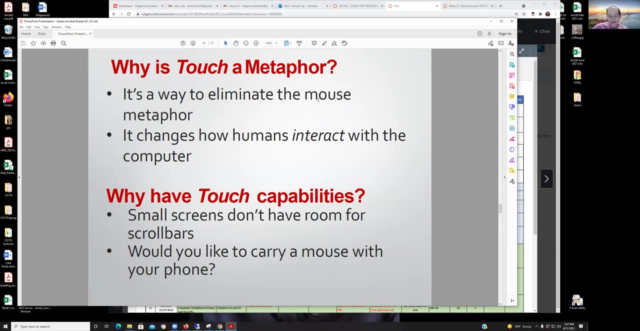 Right, everyone's kind of caught up with that, whether it's amazon, whether it's google or whatever. um, you know, we're on to touch. uh, we're doing stuff on the mobile phone, okay, all right. so basically you're transitioning from the mouse, right? that's more associated. 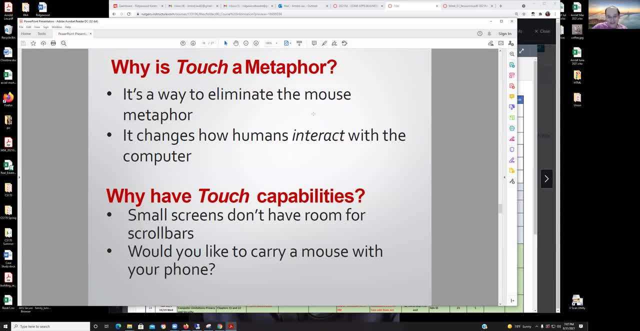 with the desktop, right, you're not really going to carry a mouse and hook it up to your phone, right? um, and you know? so this is why you went from the touch, uh, you went from the mouse to the touch, right, uh, so you have the small screen. you're not going to carry a mouse with you, stuff like that. 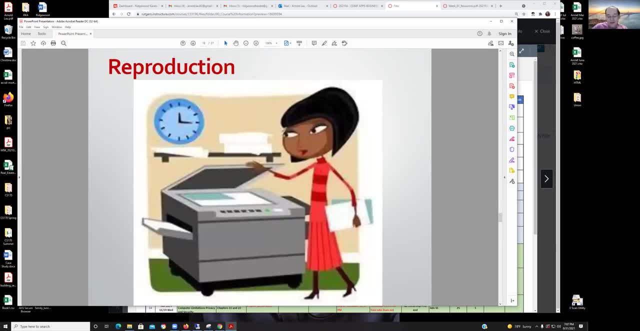 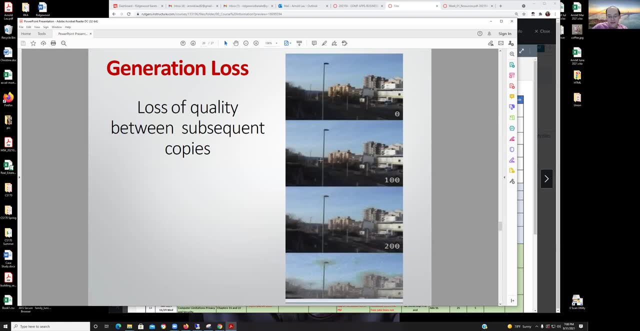 right now the reproduction. this is where we're talking about perfect reproduction, right? so this is where you know you're losing quality from one generation to another. so if you say this is your original and you go down to here, you can see how bad this looks, right? 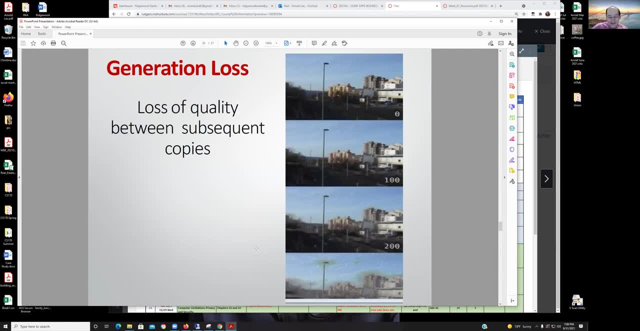 and this is what would happen if you in the old days, if you had things like records or cassette tapes or whatever, um, or you know analog pictures, essentially right, if you kept on copying it over and over again, um, you're gonna lose quality, it would degrade over time, right? so your your old movies from way back. 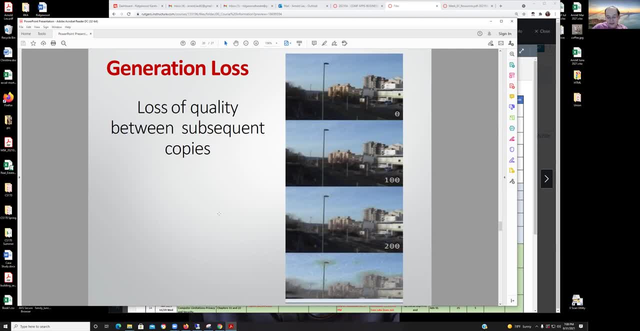 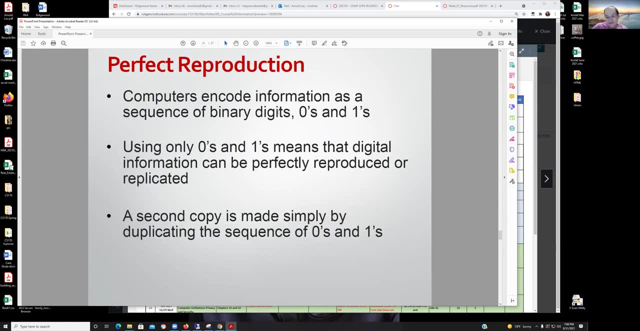 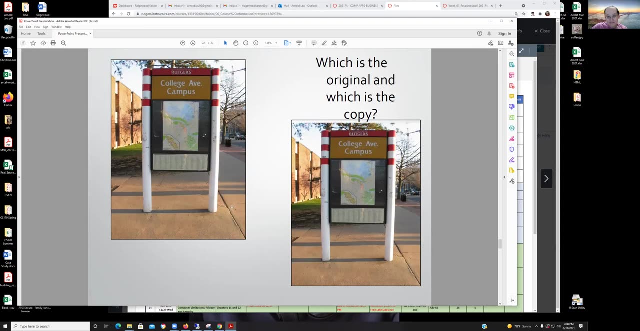 when, um, it's gonna lose quality over time because they're not stored digitally, ie, zeros and ones, right? computers store everything- zeros and ones, so you can just copy the same zeros and ones, right? okay, so this picture is the same as that picture. that's what it's meant to say, right? i don't know. 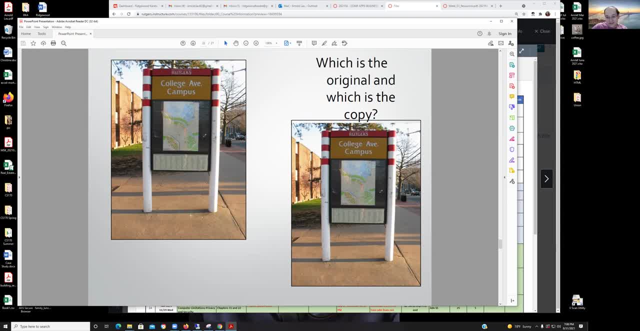 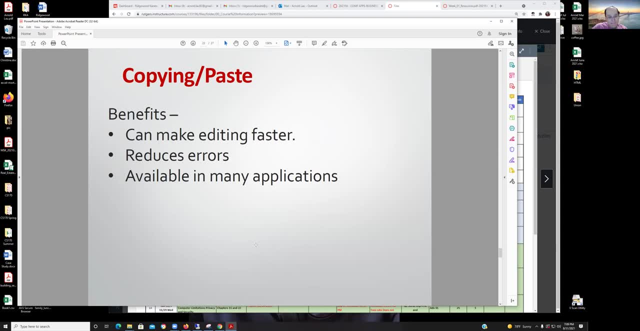 if you can really tell that looking at this. but yeah, they're supposed to be identical because you just copy one file to another, right? exact copy, okay, so copy and paste is a big thing, right? everyone, uh, everyone's probably doing a ton of copy and paste, right? uh, just don't do it for your- uh, your- homework assignments, please. okay. 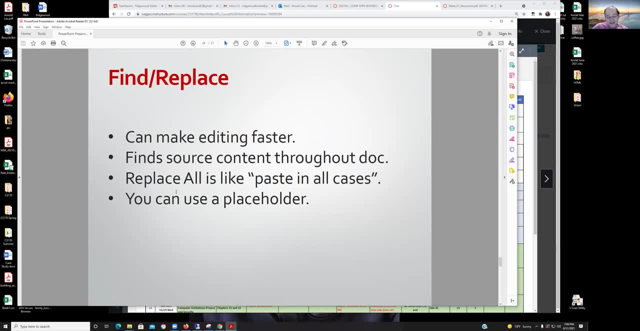 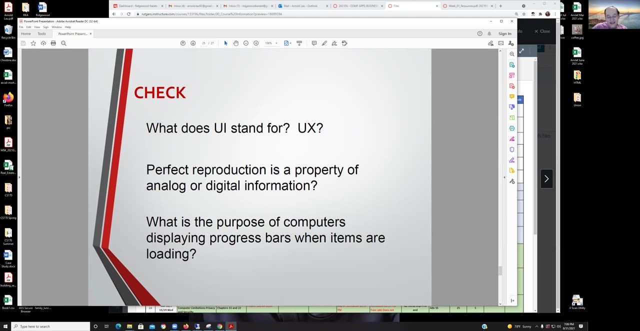 uh find and replace another type of- uh easy type of thing that you know, probably people uh do a lot of right. uh, you're editing like long a document or something like that, okay, and you know there's just like a little check in there, right? so, uh, what does ui stand for? what does ux stand for? 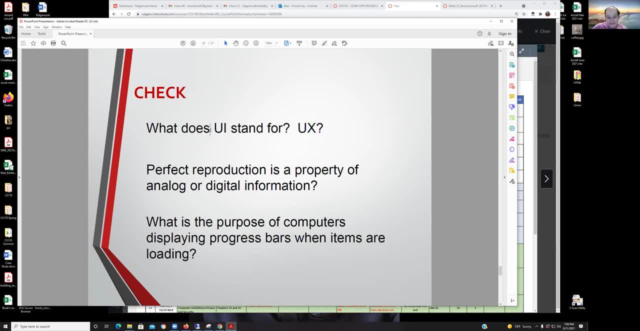 okay, um, if you don't know that, uh, make sure you look it up in the in the book, or refer back to what i said in the in the lecture. um, yeah, that should. that's those. these are important concepts here. all right, um, and then perfect reproduction. 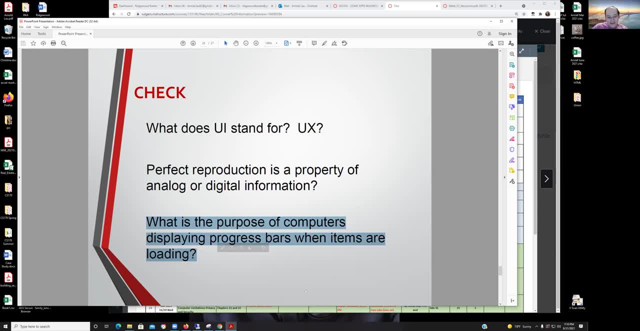 and then purpose: okay, um, this is one of those type of things. you can be pretty sure it's. we're gonna ask something like this on the exam, right, um? but i think if, uh, this concept is, you know, it shouldn't be too difficult for people to understand. but if people are not, 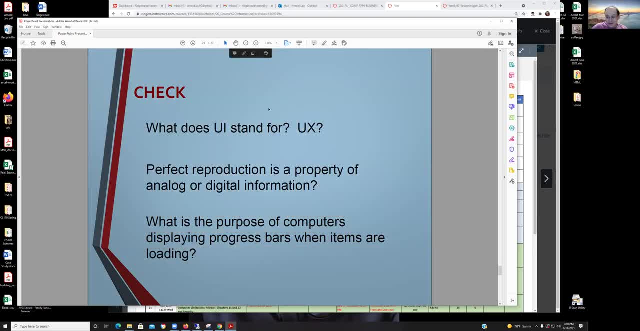 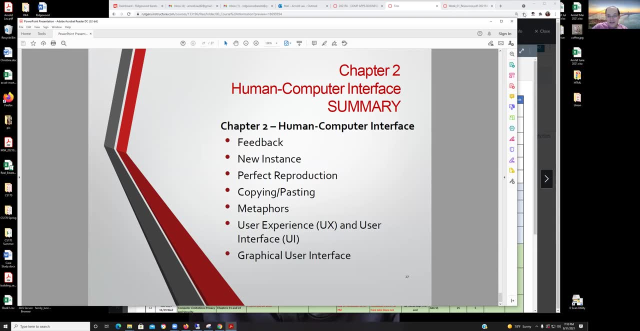 understanding that. make sure you let me know and i'll try to clarify for the next lecture. okay, all right, so i think i'll leave it at that. i'm going to upload this to my area and you'll be able to see it, okay, so hopefully this is nice and 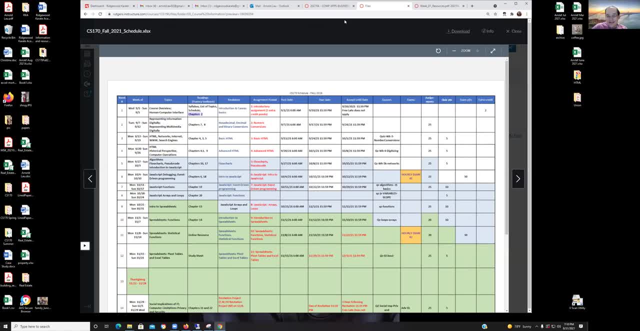 short. if there's any questions at all, just give me a shout. thank you, have a good night.